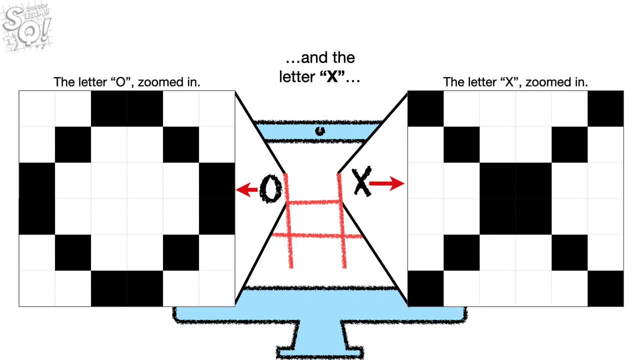 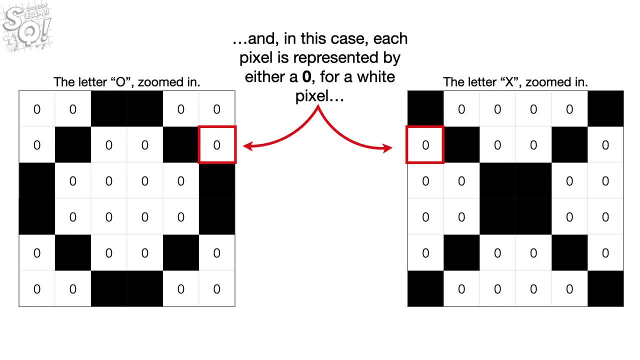 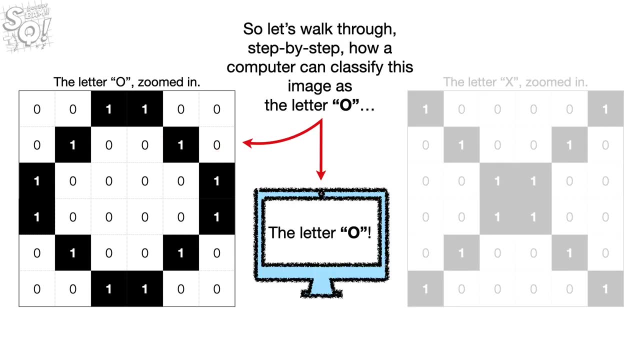 in on the letter o and the letter x and see that each image is just a bunch of pixels, And in this case, each pixel is represented by either a zero for a white pixel or a one for a black pixel. So let's walk through, step by step, how a computer can classify this image. 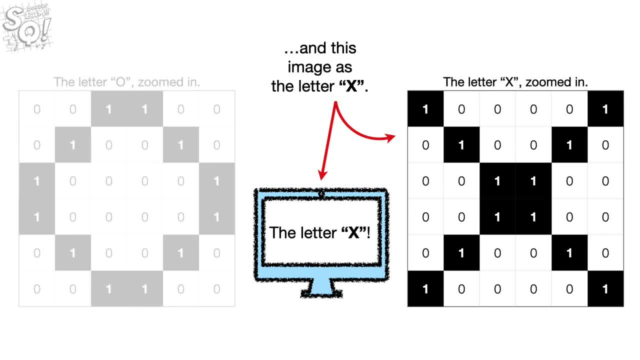 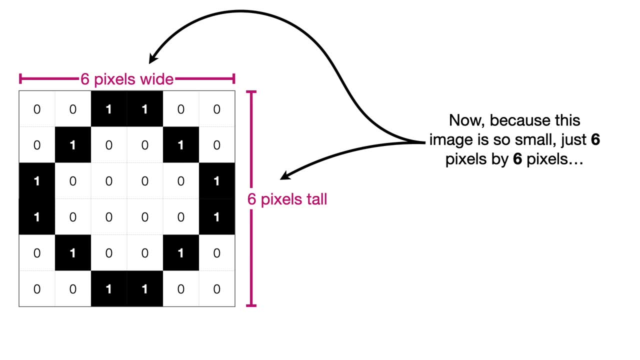 as the letter o and this image as the letter x. We will start with the image of the letter o Now, because this image is so small, just 6 pixels by 6 pixels. it is possible to make a normal everyday neural network that can. 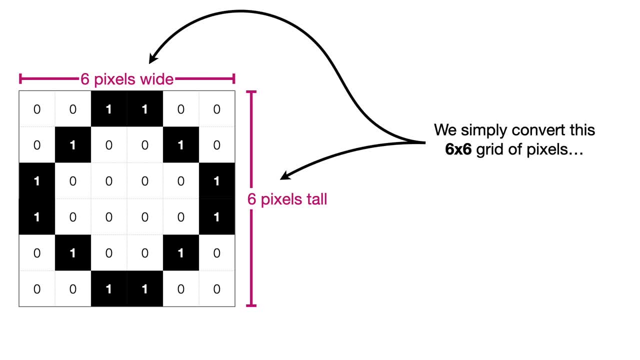 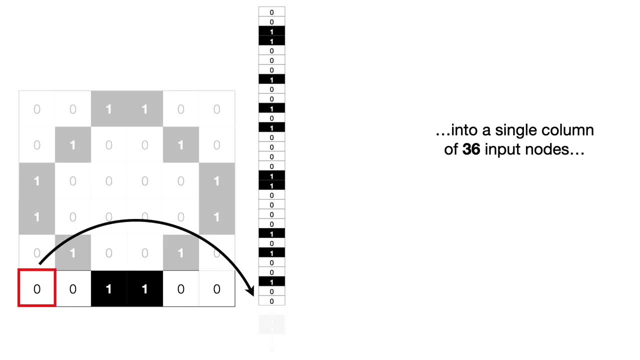 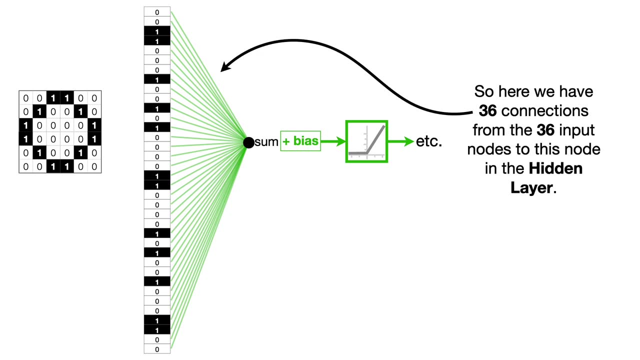 correctly classify it. We simply convert this 6 by 6 grid of pixels into a single column of 36 input nodes- Bip, bip, bip, Bip, bip, bip- And connect the input nodes to a hidden layer. So here we have 36 connections from the 36 input nodes to this node in the hidden layer. 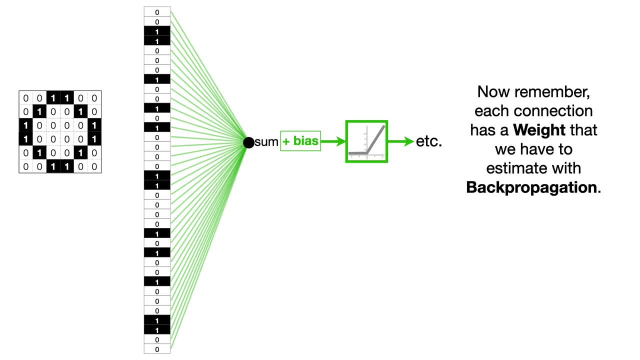 Now remember: each connection has a weight that we have to estimate with backpropagation. So that means we need to estimate 36 weights in order to connect to this node. However, usually the first hidden layer has more than 1 node. Bip, bip, bip. 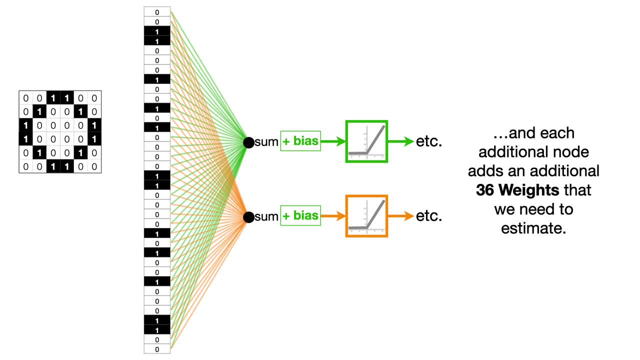 Bip, bip. Each additional node adds an additional 36 weights that we need to estimate, Like I said, because the original image is small- 6x6, and black and white. something like this could work, However, if we had a larger image, like 100 pixels by 100 pixels, which is still pretty. 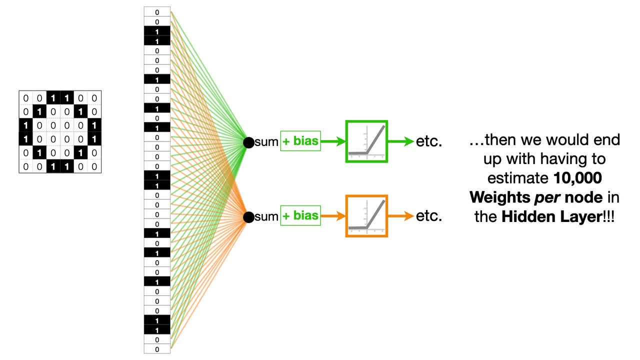 small compared to real world pictures. then we would end up having to estimate 10,000 weights per node in the hidden layer, So this method doesn't scale very well. Another problem is that it's not clear that this neural network will still perform well. 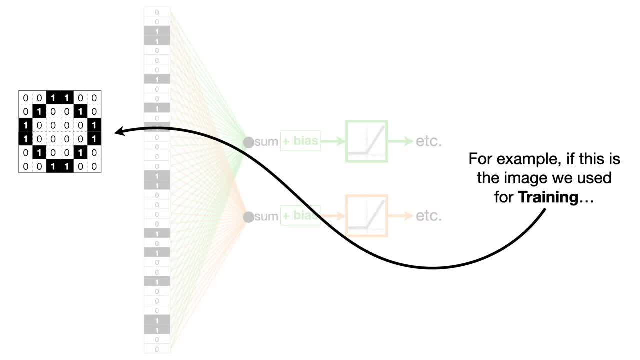 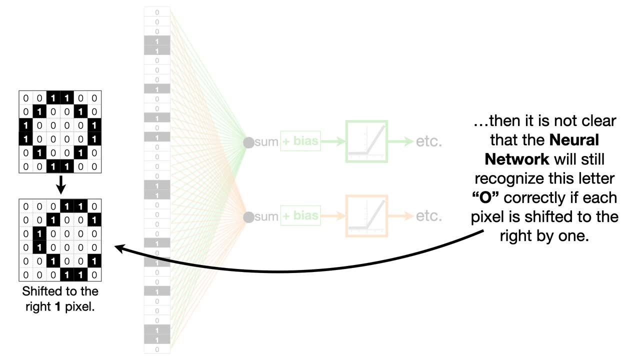 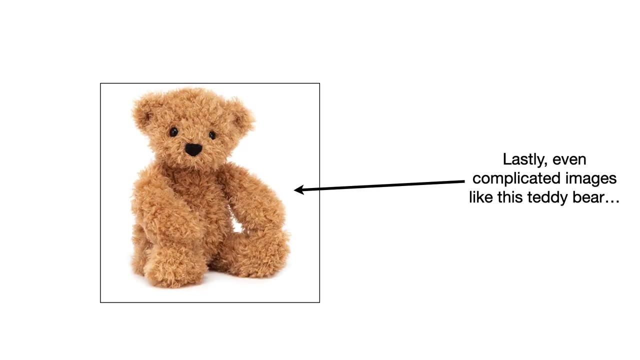 if the image is shifted by one pixel. For example, if this is the image we used for training, then it is not clear that the neural network will still recognize this letter O correctly if each pixel is shifted to the right by one. Lastly, even complicated images like this teddy bear will still perform well if the 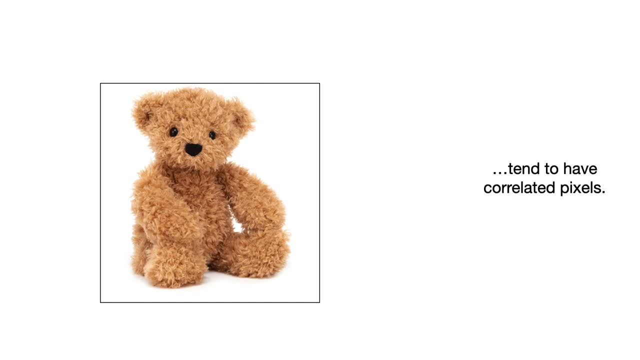 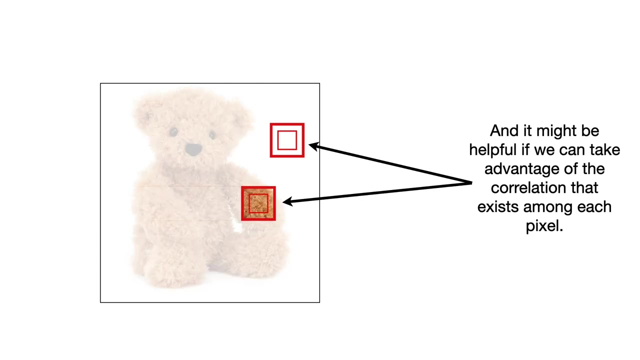 image is shifted to the left by one pixel. For example, any brownish pixel in this image tends to be close to other brown pixels And any white pixel tends to be near other white pixels, And it might be helpful if we can take advantage of the correlation that exists among each. 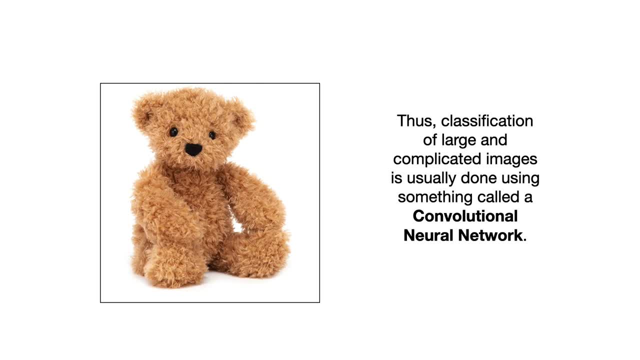 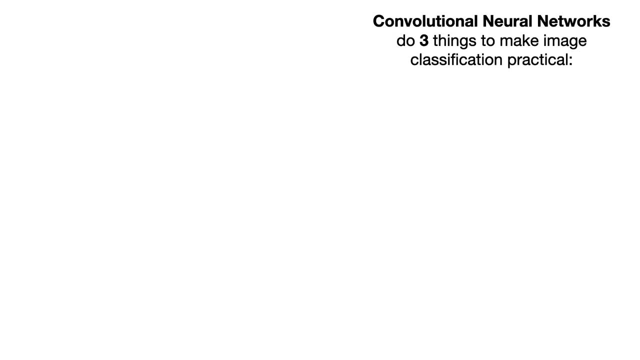 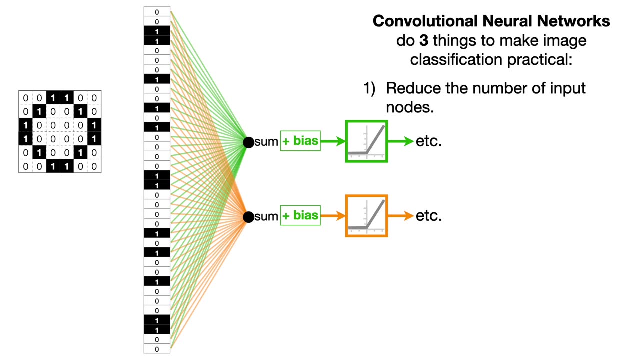 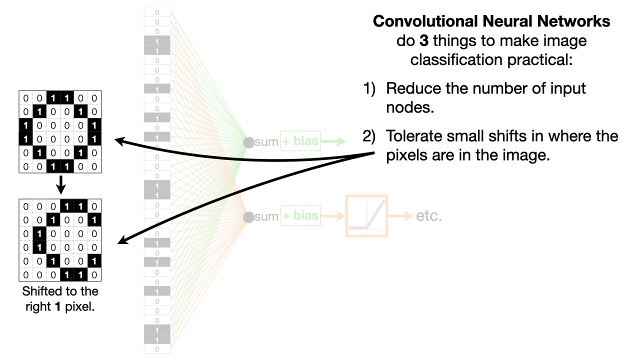 pixel. Thus, classification of large and complicated images is usually done using something called a convolutional neural network. Convolutional neural networks do three things to make image classification practical. One, they reduce the number of input nodes. Two, they tolerate small shifts in where the pixels are in the image. 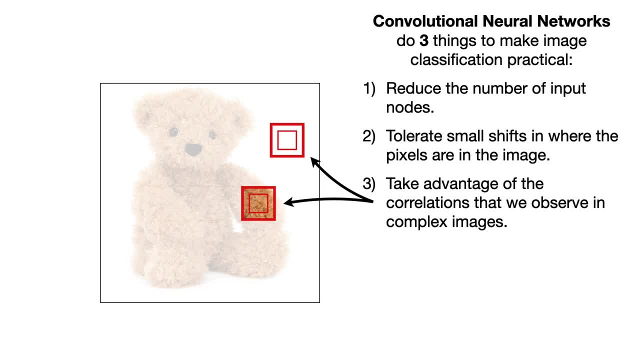 And three take advantage of the correlations that we observe in complex images. So let's go back to our tic-tac-toe game. 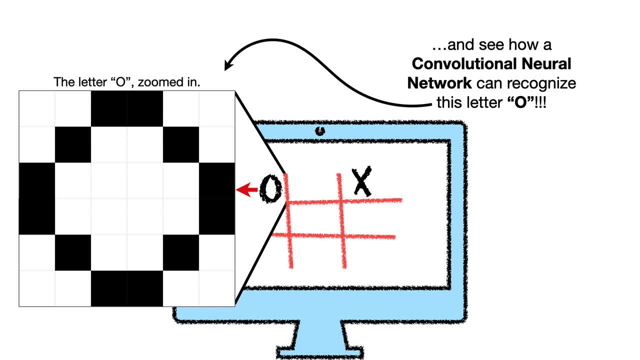 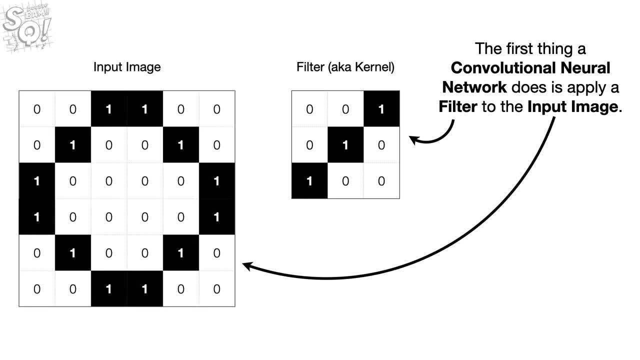 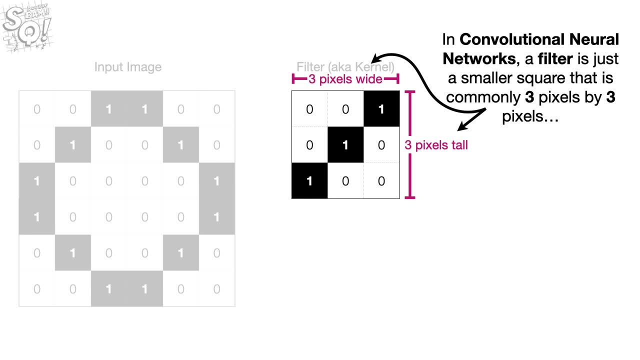 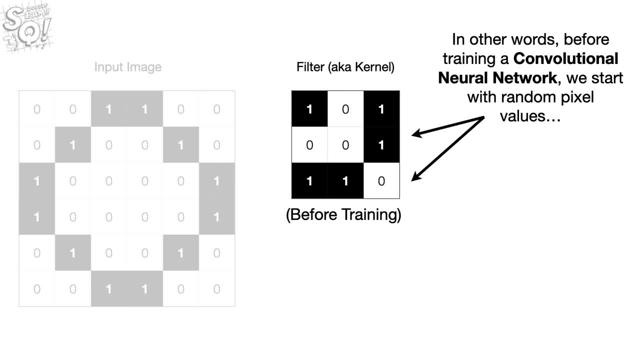 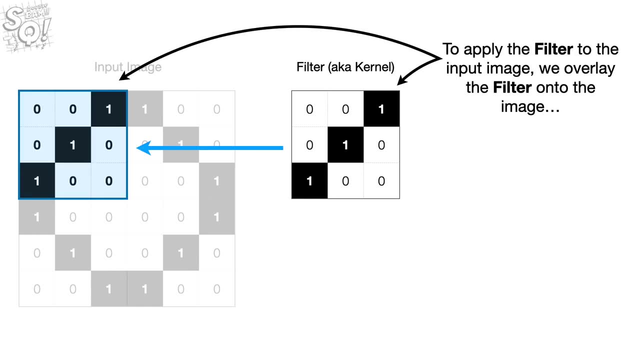 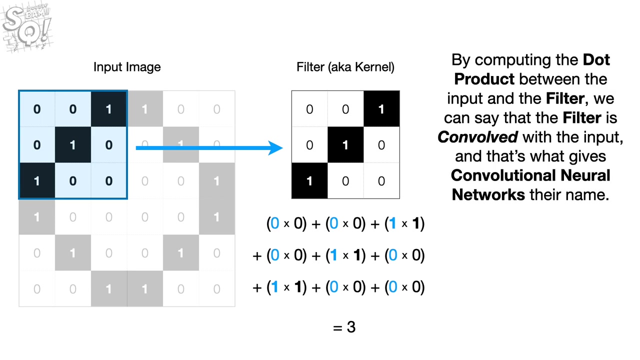 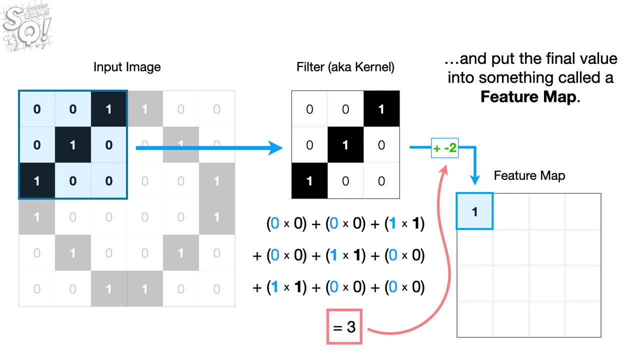 Now, in this example we slide the filter over one pixel. However, other convolutional neural networks might move over two or more pixels, But in this example we just move over one pixel. 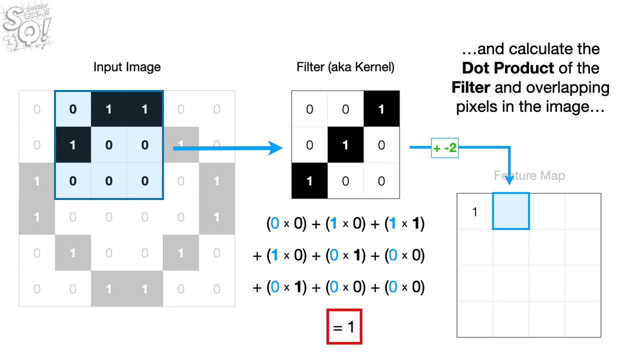 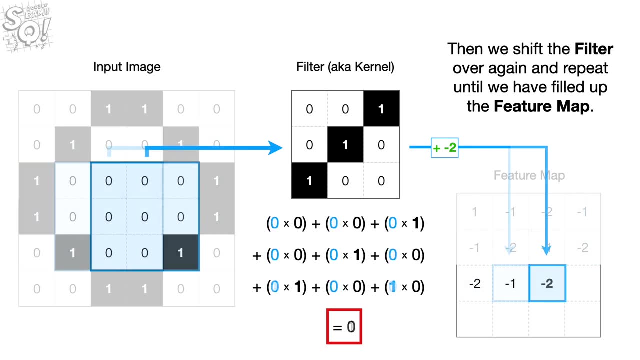 And calculate the dot product of the filter and overlapping pixels in the image, Add the bias term And put the final value into the feature map. Then we shift the filter over again And repeat until we have filled up the feature map. Bip, Bip, Bip, Bip, Bip, Bip, Bip. 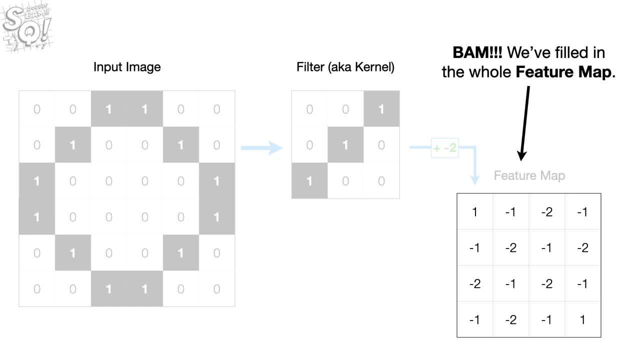 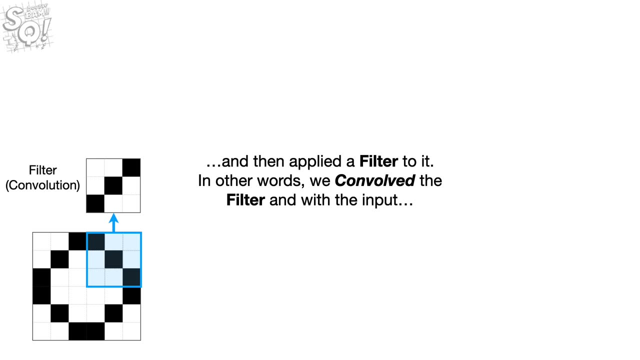 Bam. We filled up the whole feature map. To summarize, we started with an input image of the letter O And then applied a filter to it. In other words, we convolved the filter with the input And added a bias term to the values. 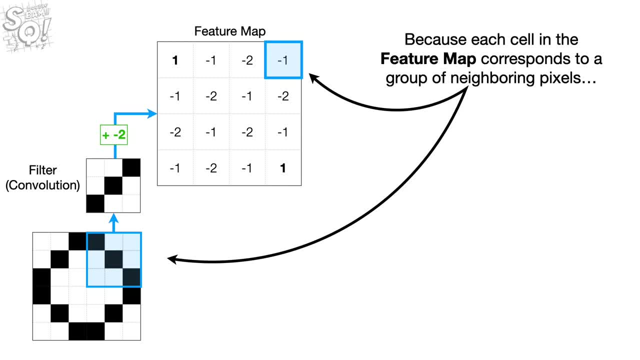 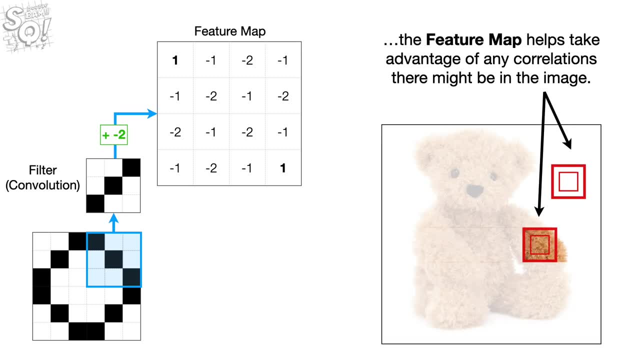 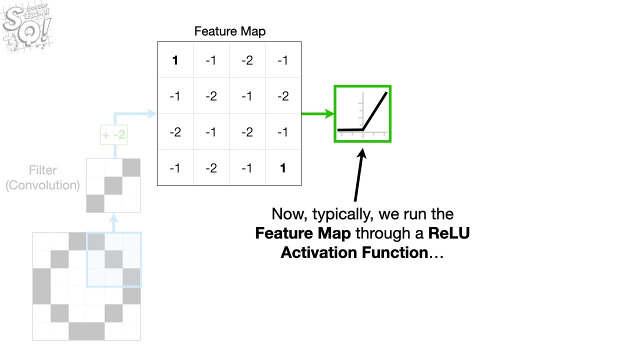 And that gave us a feature map. Because each cell in the feature map corresponds to a group of neighboring pixels, the feature map helps take advantage of any correlations there might be in the image Bam. Now, typically we run the feature map through a relu activation function. 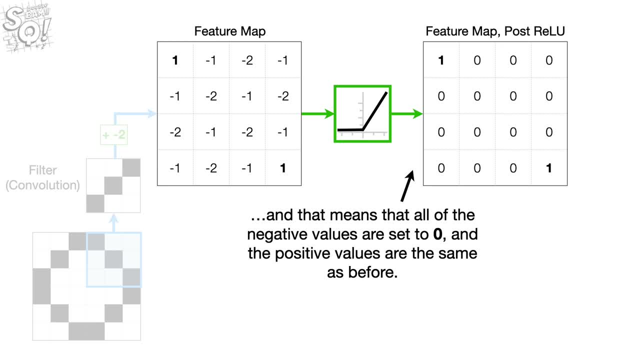 And that means that all of the negative values are set to 0.. And the positive values are the same as before. In this case, that means everything gets set to 0.. before. In this case, that means everything get set to 0.. 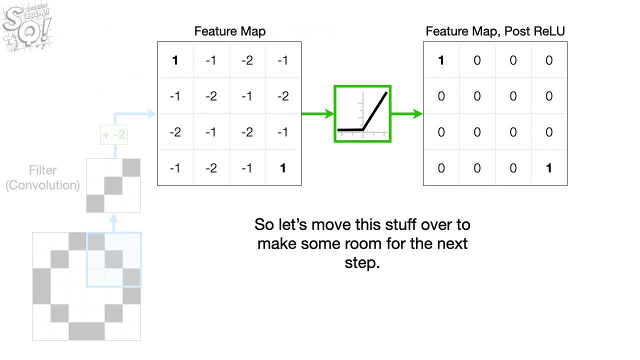 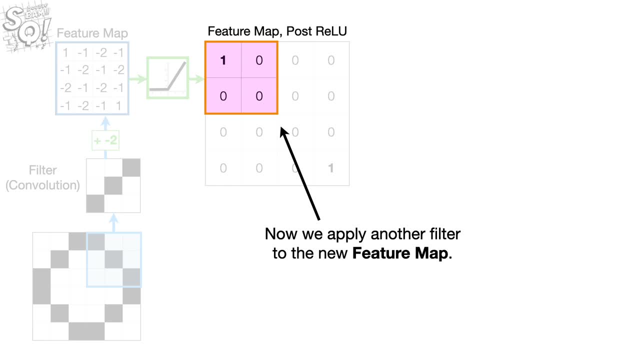 0.. in this case, that means everything gets set to 0. except for these two points. So let's move this stuff over to make some room for the next step. Now we apply another filter to the new feature map. However, unlike before, 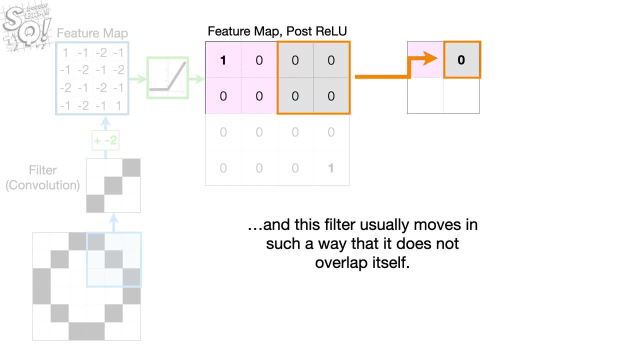 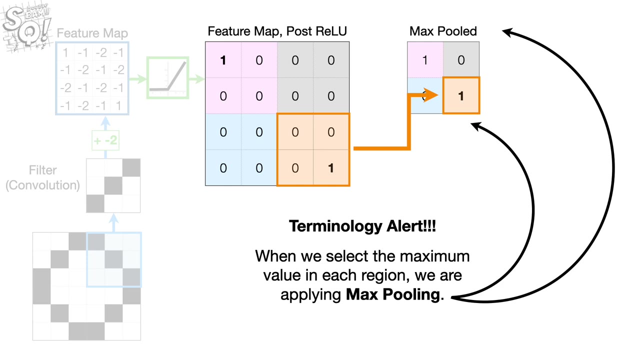 we simply select the maximum value And this filter usually moves in such a way that it does not overlap itself. Oh no, it's another dreaded terminology. alert: When we select the maximum value in each region, we are applying max pooling. To see the effect that max pooling has in this example: 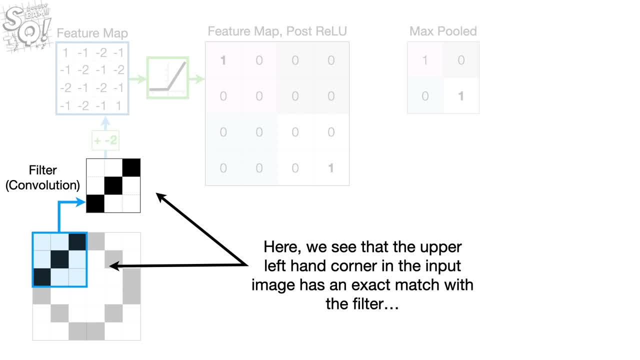 let's go back to the input image. Here we see that the upper left-hand corner in the input image has an exact match with the filter And this results in the highest possible value in the feature map. And then the max pooling step reduce this region. 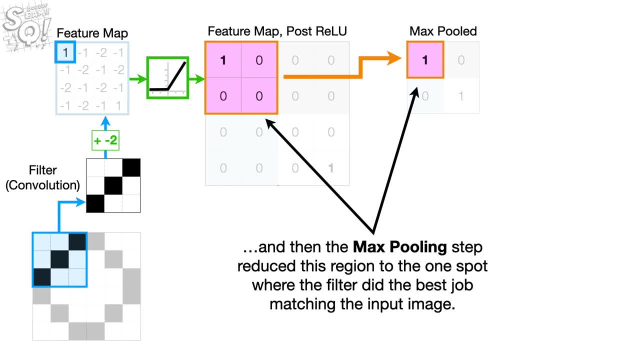 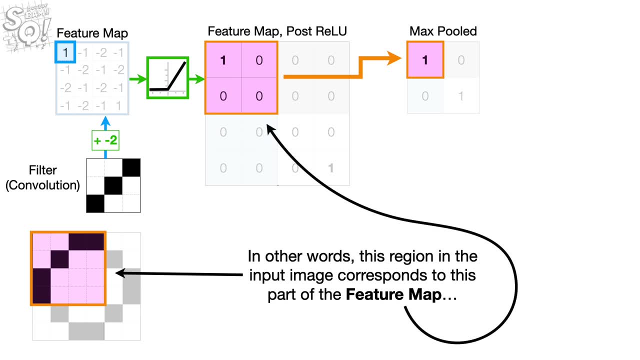 to the one spot where the filter did the best job matching the input image. In other words, this region in the input image corresponds to this part of the feature map And the max pooling step selected the spot where the filter did the best job matching the input image. 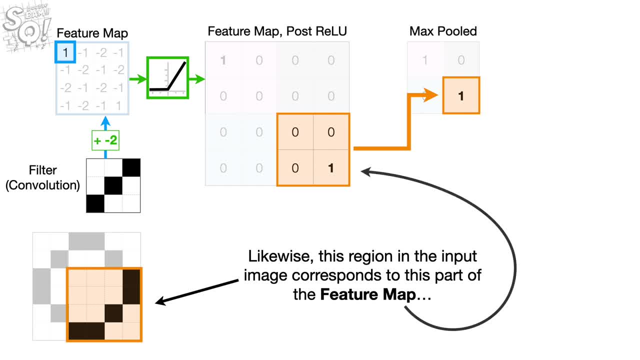 Likewise, this region in the input image corresponds to this part of the feature map And the max pooling step selected the spot where the filter did the best job, matching the input image. So we see that max pooling selects the spots where the filter did the best job. 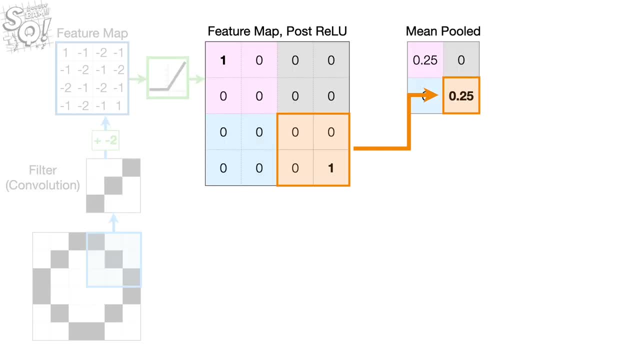 matching the input image. Oh no, it's another terminology alert. Alternatively, we could calculate the average value for each region, and that would be called average or mean pooling. Now, going back to the max pooled layer, let's move and shrink things to give us more room. 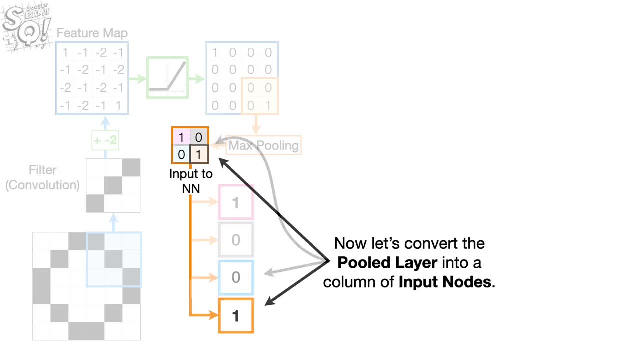 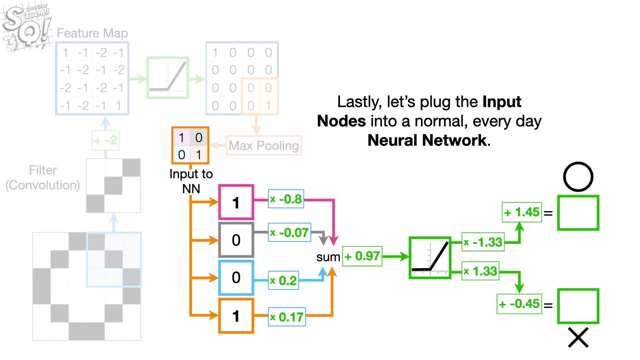 Now let's convert the pooled layer into a column of input nodes. Lastly, let's plug this in. Let's plug the input nodes into a normal, everyday neural network. This neural network has four input nodes: a single hidden layer with a single node. 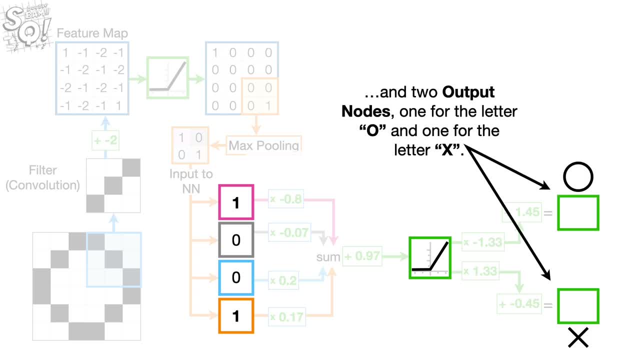 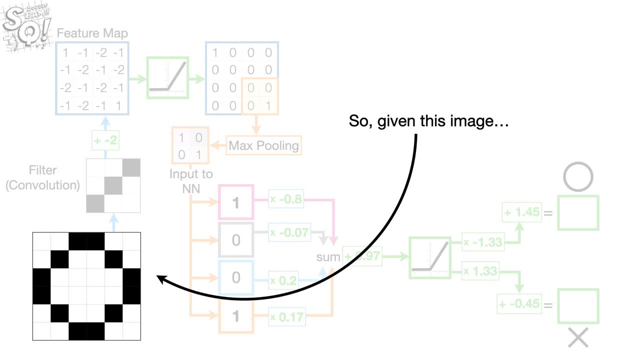 using the relu activation function and two output nodes, one for the letter O and one for the letter X. So, given this image, we run it through the filter to create the feature map, Then we run the feature map through a relu activation function, then we select the maximum value in each area. 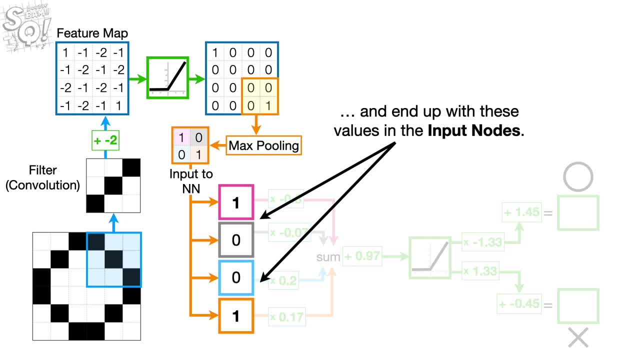 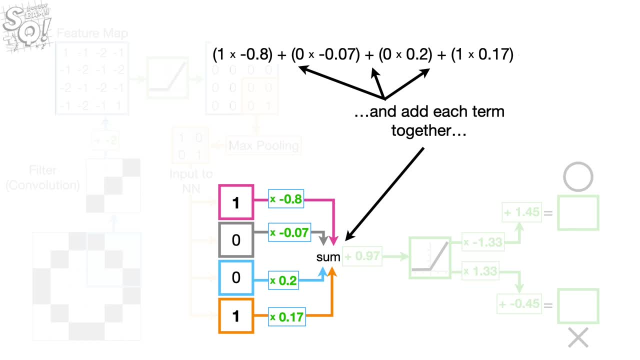 and end up with these values in the input nodes. Now we multiply the values in the input nodes by their associated weights and add each term together, And then add the bias and we end up with 0.34.. And thus the X-axis coordinate. 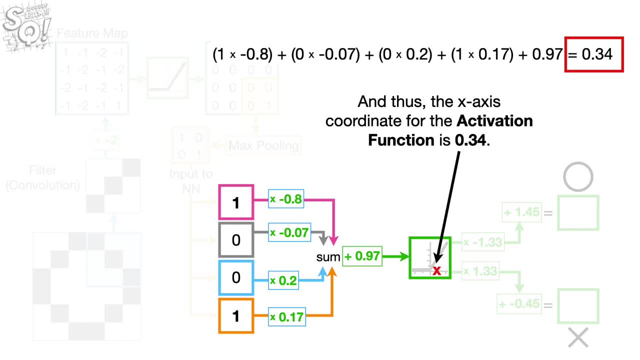 for the activation function is 0.34.. Now we plug 0.34 into the relu activation function and the output is 0.34, because 0.34 is greater than 0. Now this connection from the hidden layer to the output for the letter O. 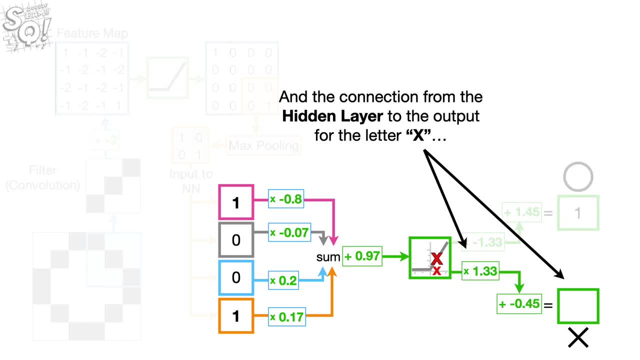 gives us 1 for the letter O And the connection from the hidden layer to the output for the letter X gives us 0 for the letter X. So when the input is 0, and the input is a picture of the letter O, 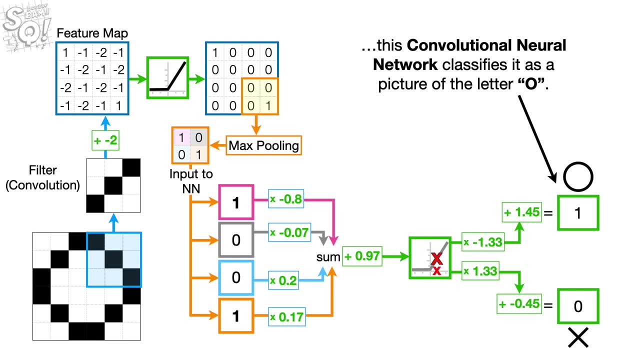 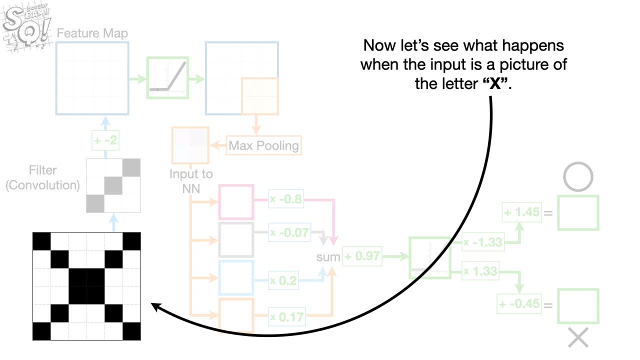 this convolutional neural network classifies it as a picture of the letter O Bam. Now let's see what happens when the input is a picture of the letter X. Note: even though we have changed the input, the filter is the same as before. 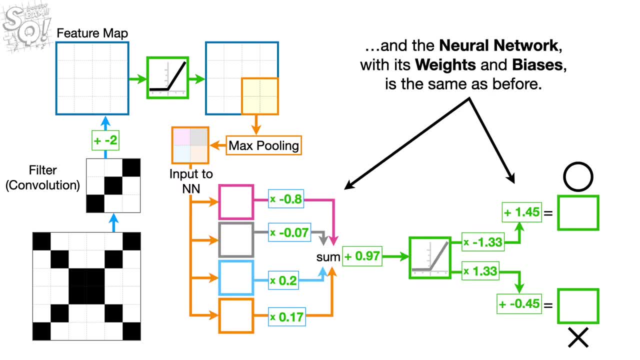 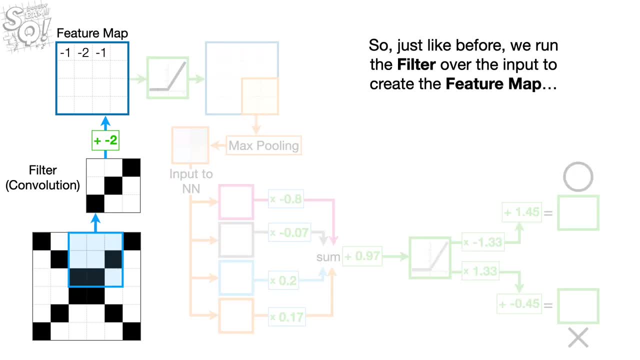 And we're doing max pooling just like before, And the neural network with its weights and biases is the same as before. So, just like before, we run the filter over the input to create the feature map. Now we run the feature map through the relu. 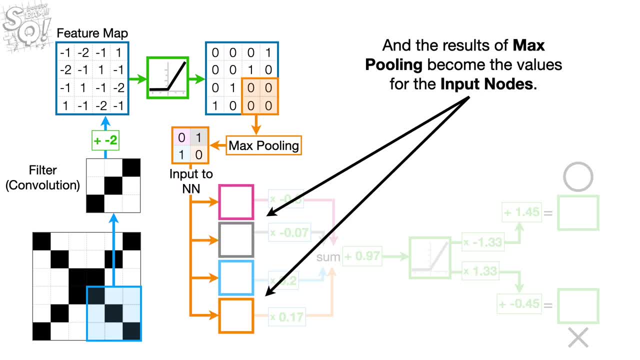 and do max pooling, And the results of max pooling become the values for the input nodes. Now we run the values in the input nodes through the neural network and the result is 0 for the letter O and 1 for the letter X. So when the input is a picture of the letter X, 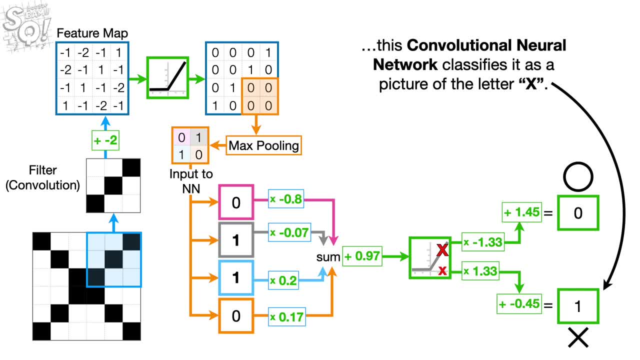 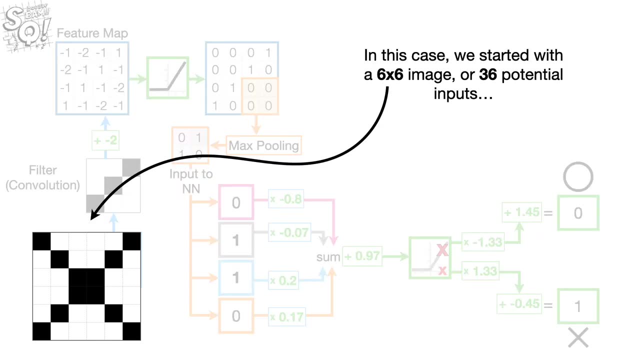 this convolutional neural network classifies it as a picture of the letter X, Double bam. Now remember that we said: convolutional neural networks help reduce the number of inputs in the neural network. In this case, we started with a 6x6 image. 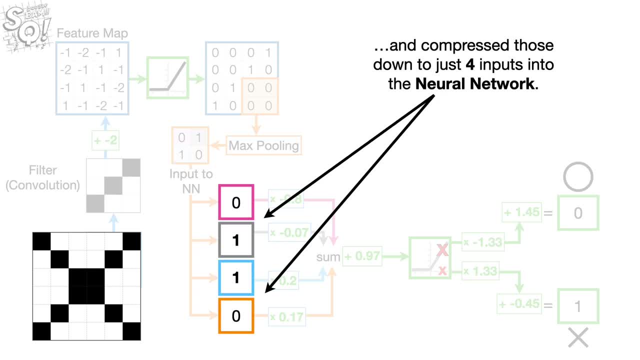 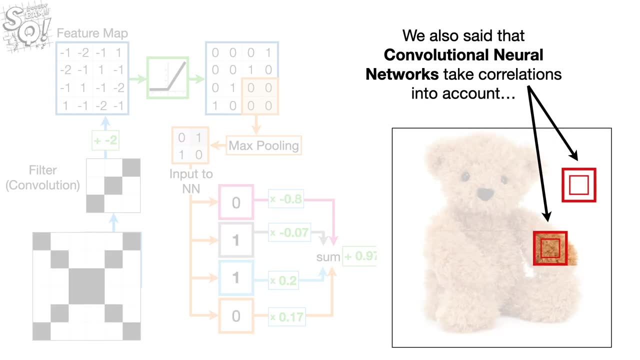 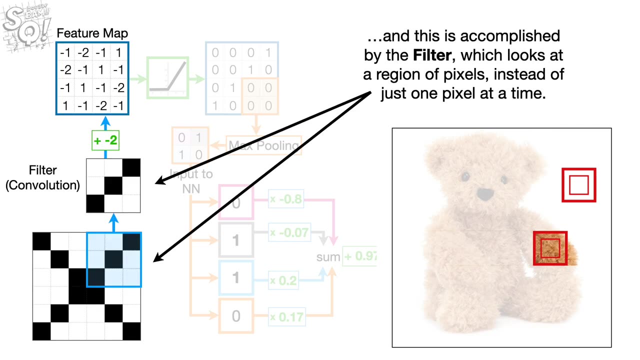 or 36 potential inputs And compress those down to just 4 inputs into the neural network. We also said that convolutional neural networks take correlations into account, And this is accomplished by the filter which looks at a region of pixels instead of just one at a time. 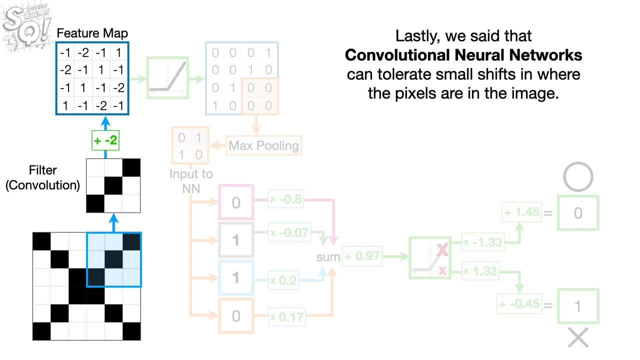 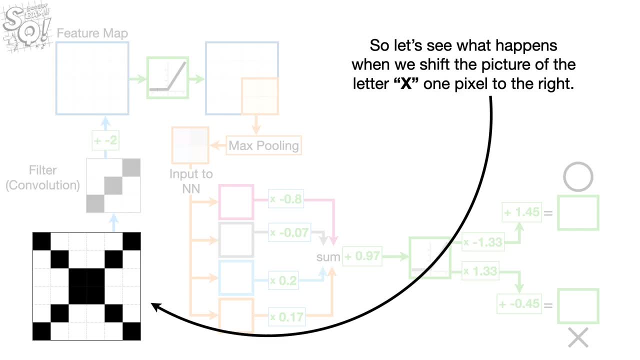 Lastly, we said that convolutional neural networks can tolerate small shifts in where the pixels are in the image. So let's see what happens when we shift the picture of the letter X one pixel to the right. In other words, will this convolutional neural network 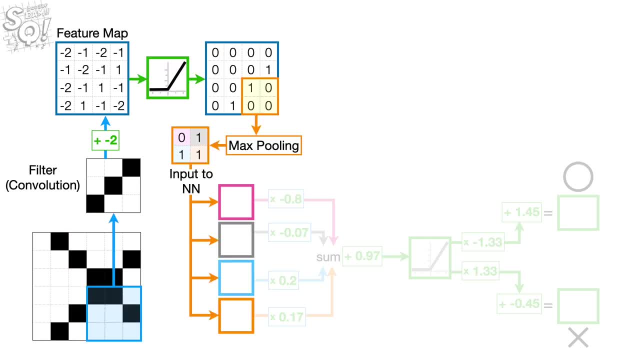 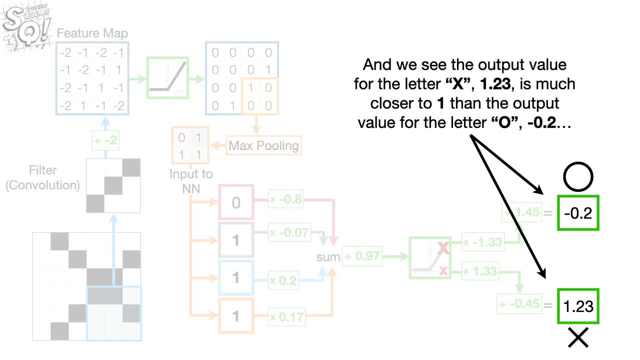 still decide if the input is a picture of the letter X And we see that the output value for the letter X- 1.23, is much closer to 1 than the output value for the letter O negative 0.2.. 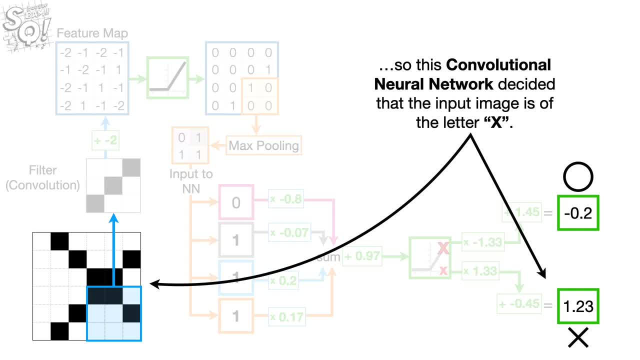 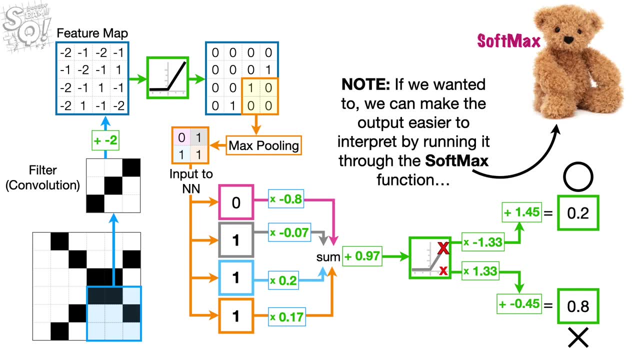 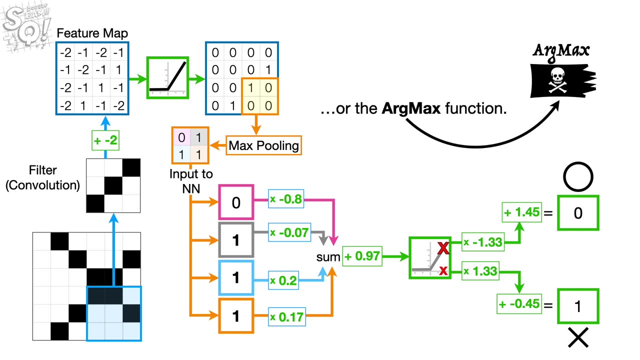 So this convolutional neural network decided that the input image is of the letter X. Well, bam Note. if we wanted to, we can make the output easier to interpret by running it through the softmax function or the argmax function, Also note. 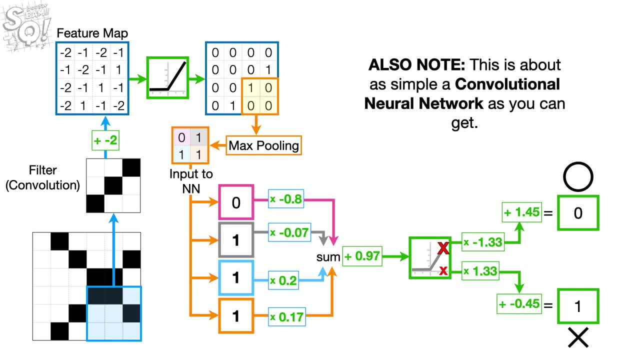 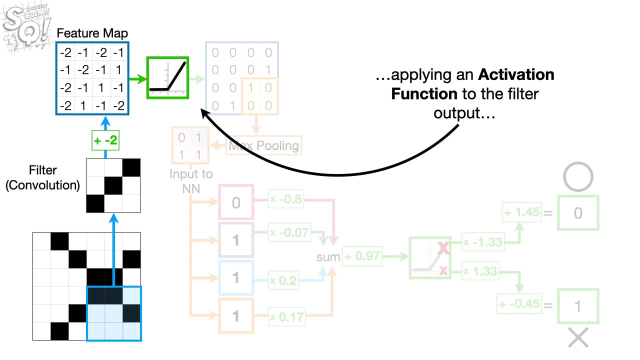 this is about as simple a convolutional neural network as you can get. However, no matter how fancy the convolutional neural network is, it's still based on filters, aka convolution: applying an activation function to the filter output and pooling the output. 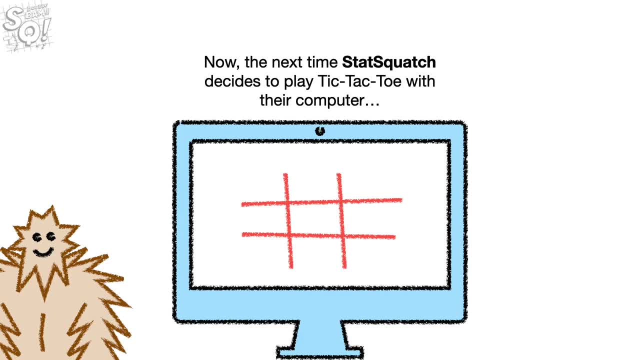 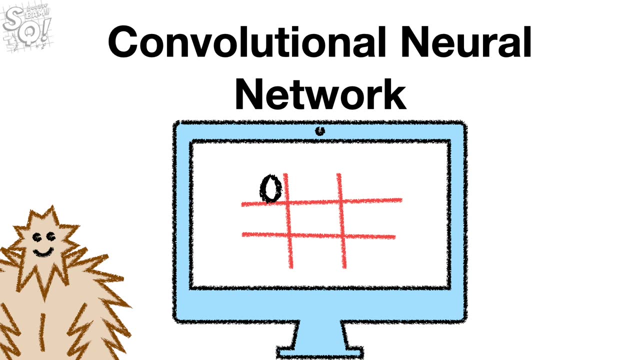 of the activation function. Now, the next time Statsquatch decides to play tic-tac-toe with their computer, Statsquatch can start with the letter X or the letter O and a convolutional neural network. We'll figure it out. 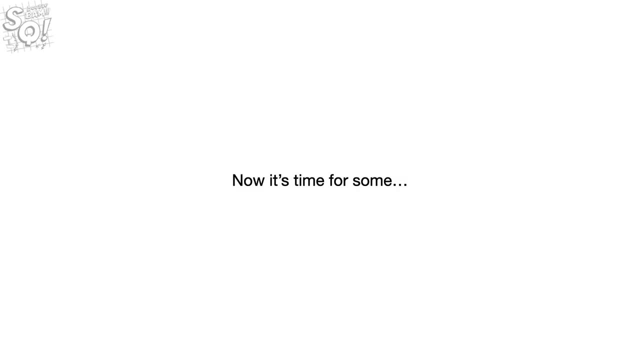 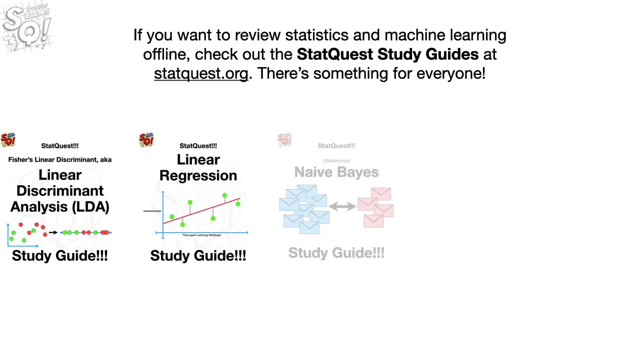 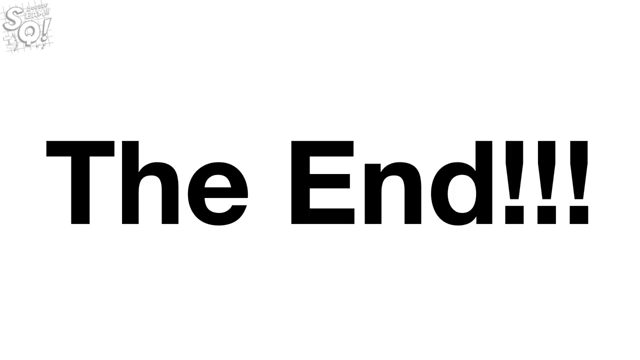 Bam. Now it's time for some shameless self-promotion. If you want to review statistics and machine learning offline, check out the StatQuest study guides at statquestorg. There's something for everyone. Hooray, We've made it to the end of another exciting StatQuest.